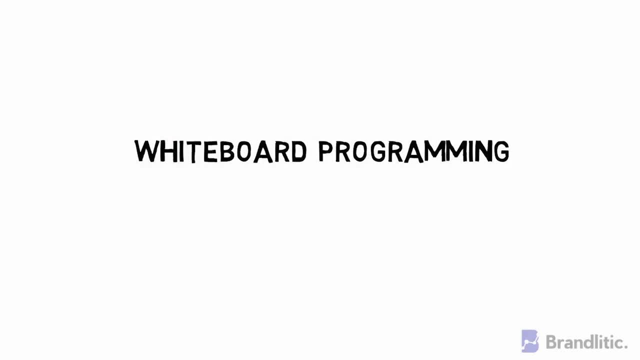 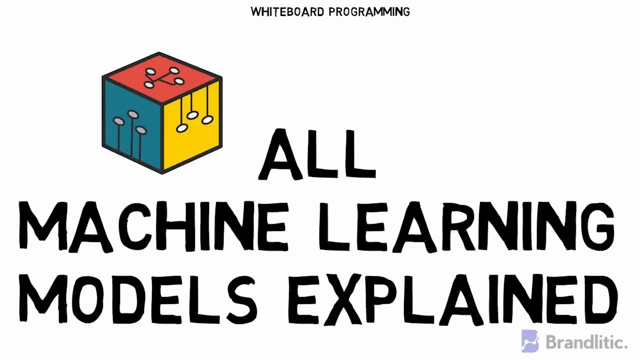 Welcome to Whiteboard Programming, where we simplify programming for you with easy-to-understand whiteboard videos, And today I'll be giving you a brief explanation of all machine learning models. So let's get started. Broadly speaking, all machine learning models can be categorized as supervised or unsupervised. 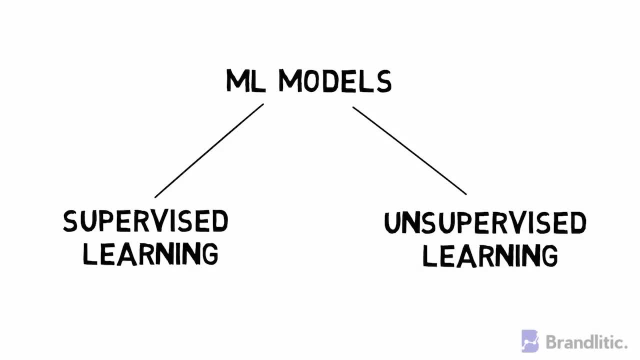 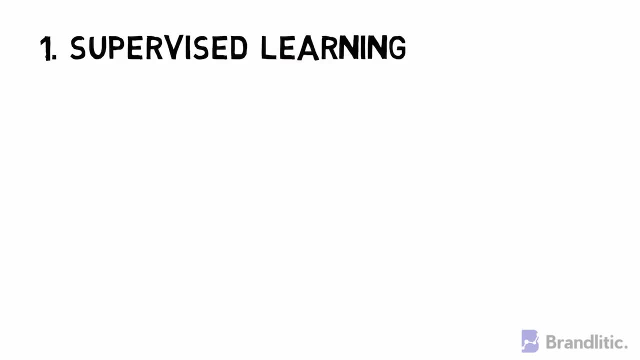 We'll uncover each one of them and what all types they have. 1. Supervised Learning: It involves a series of functions that map an input to an output based on a series of example: input-output pairs. For example, if we have a dataset of two variables, one being 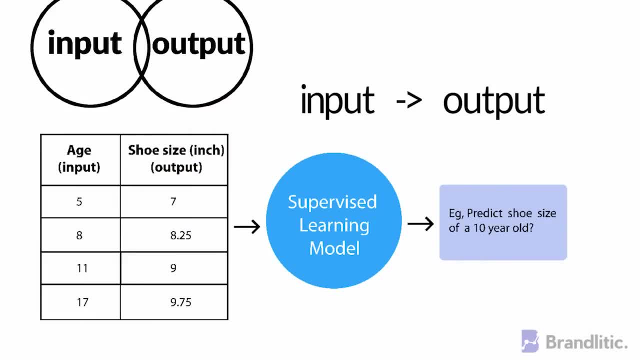 age, which is the input, and other being the shoe size as output, we could implement a supervised learning model to predict the shoe size of a person based on their age. Further, with supervised learning, there are two subcategories: One is regression and the 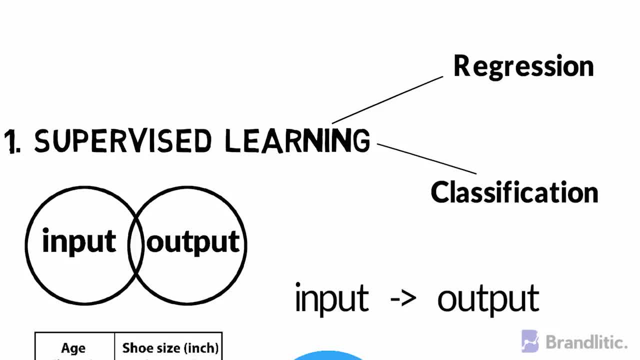 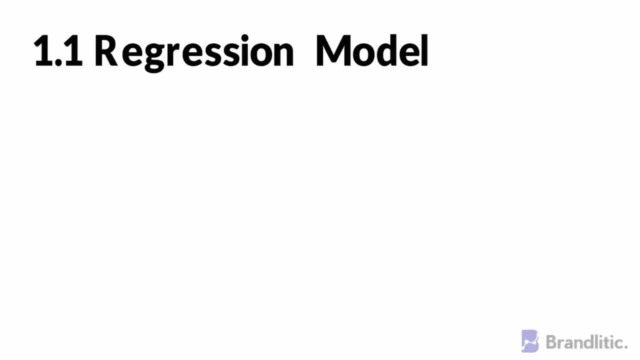 other is classification. In Regression Model, you can find a target value based on independent predictors. That means you can use this to find a relationship between a dependent variable and an independent variable. In regression models, the output is continuous. Some of the most common types of regression models include: 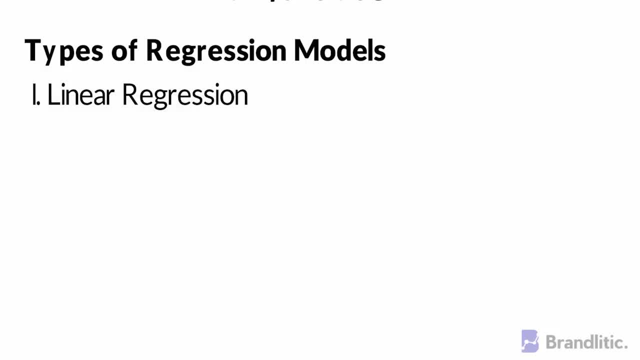 1. Linear Regression, Which is simply finding a line that fits the data. Its extensions include multiple linear regression, that is finding a plane of best fit, and polynomial regression, that is finding a curve for best fit. 2. Decision Tree: 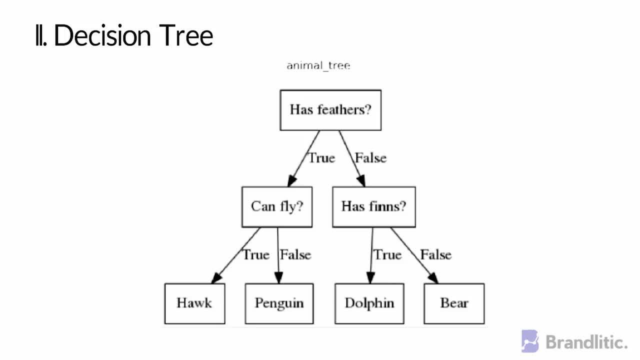 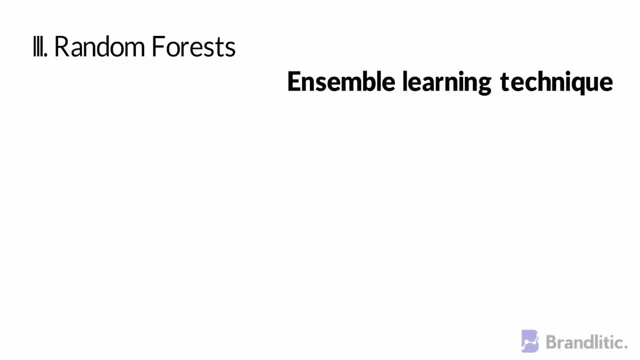 It looks like this, where each square above is called a node 3.. Random Forest: These are ensemble learning techniques that builds off of the decision trees and includes multiple decision trees, using bootstrapped dataset of original data and randomly selecting a subset of variables at each step of the revision. 4. General Training: As an instructor, here I can see that everyone is applying the exact Qui from all the data 類 of the line. she already knows and thinks this goes the best to her. 5. Autonomy Nabemos, studing From the analysis studyletters cannot say much about the 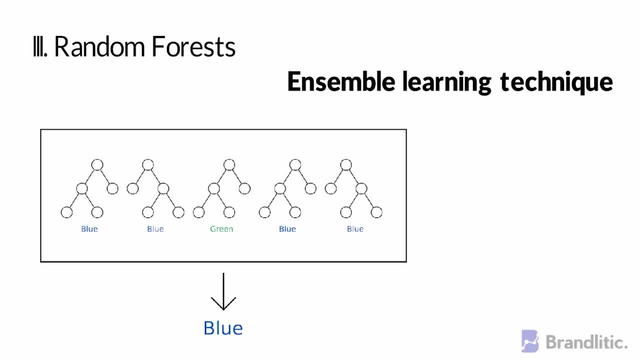 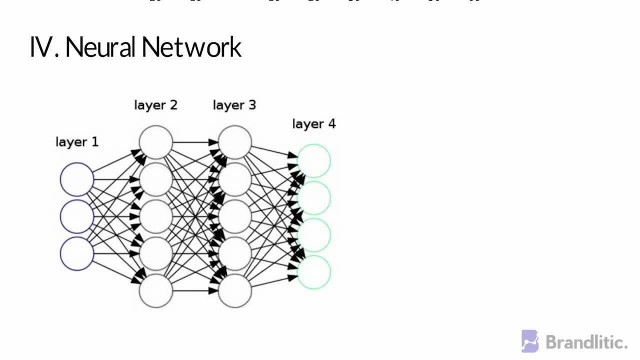 step of the decision tree. the model then selects the mode of all the predictions of each decision trees and by relying on the majority wins model, it reduces the risk of error from individual tree. next, neural network. it is quite popular and is a multi-layered model inspired by human mind. 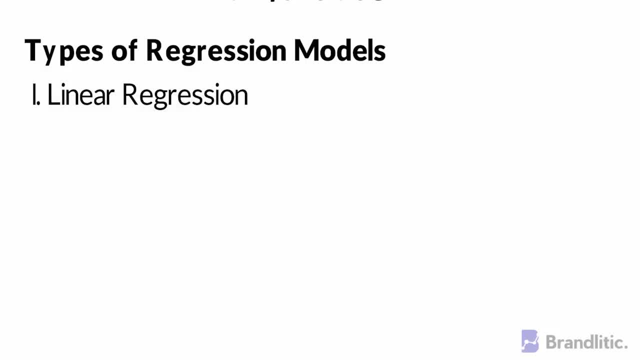 1. Linear Regression, Which is simply finding a line that fits the data. Its extensions include multiple linear regression, that is finding a plane of best fit, and polynomial regression, that is finding a curve for best fit. 2. Decision Tree: 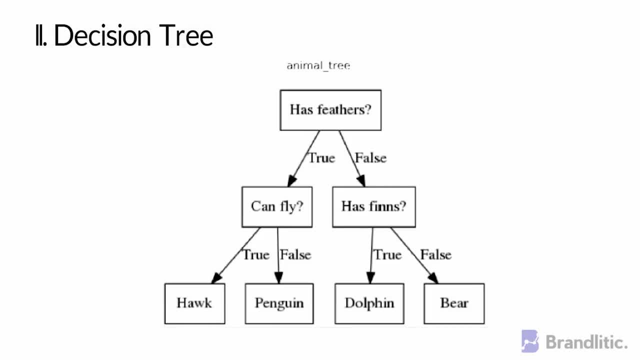 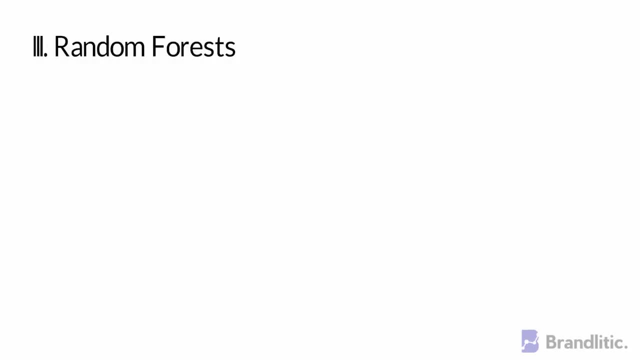 It looks something like this, where each square above is called a node, and the more nodes you have, the more accurate your decision tree will be in general. 3. Random Forest: These are assembled learning techniques that builds off decision trees and involve creating. 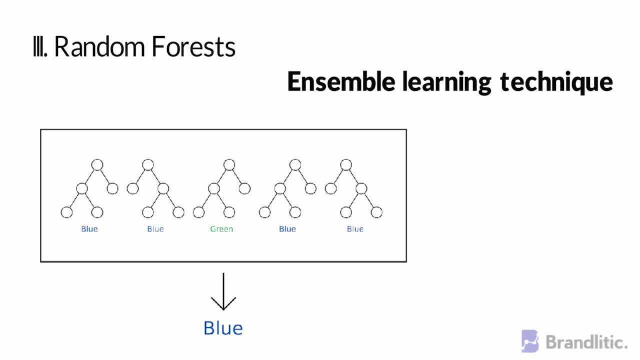 multiple decision trees using bootstrap datasets of original data and randomly selecting a subset of variables at each step of the process. 4. Random Forest- step of the decision tree. the model then selects the mode of all the predictions of each decision trees and, by relying on the majority wins model, it reduces the 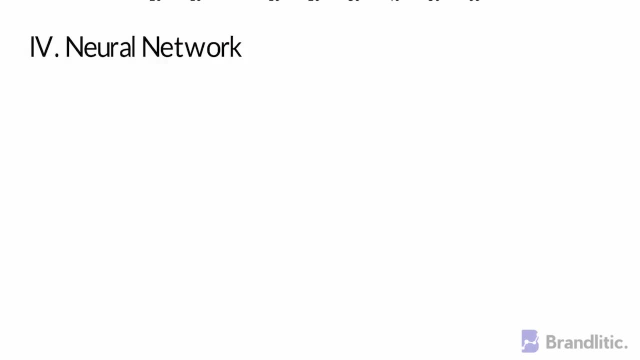 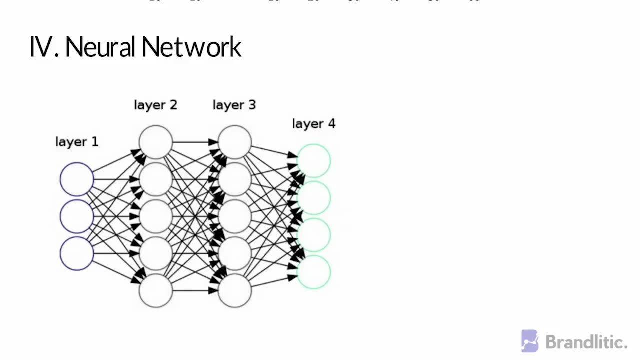 risk of error from individual tree. next, neural network. it is quite popular and is a multi-layered model inspired by human mind, like the neurons in our brain. the circle represents a node, the blue circle represents an input layer, the black circle represents a hidden layer and the green circle represents the. 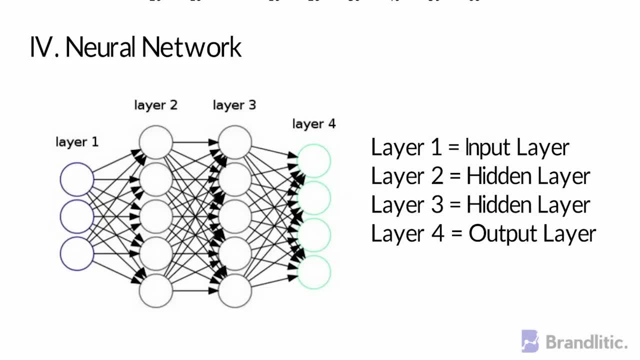 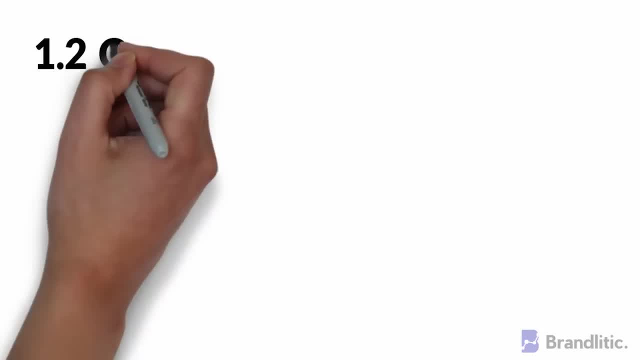 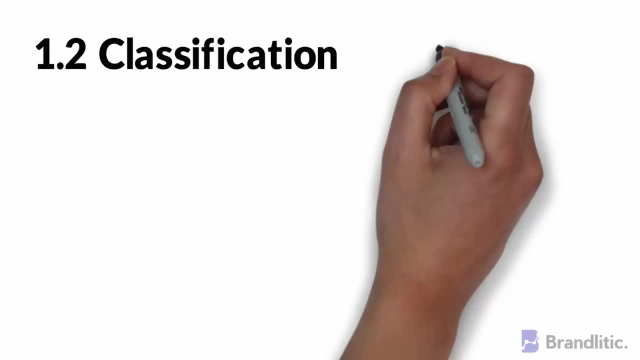 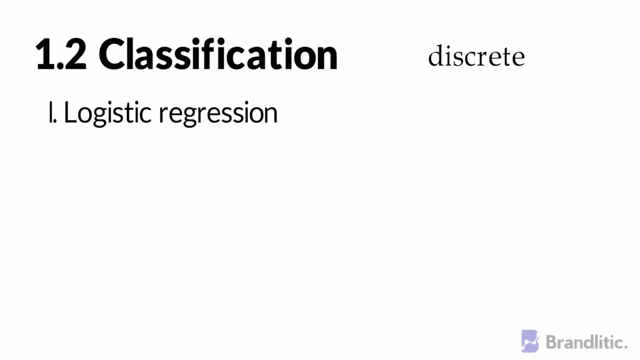 output layer. each node in the hidden layer represents a function that input goes through, ultimately leading to the output in the green circles. next classification. so with regression types being over now, let's jump to classification. so in classification, the output is discrete. some of the most common types of classification models include, first, logistic regression, which 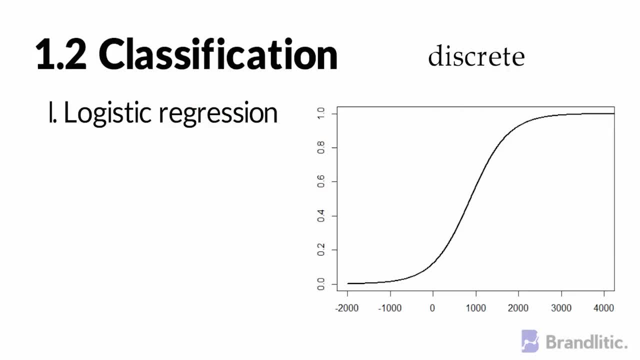 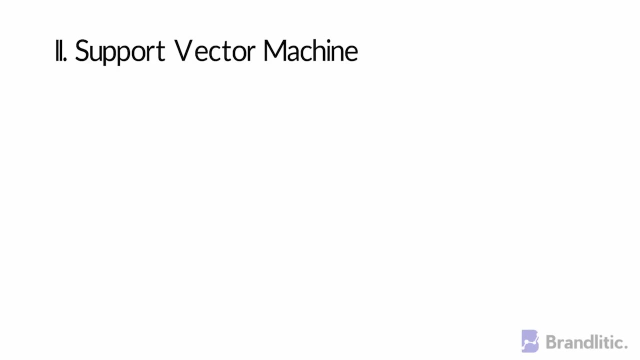 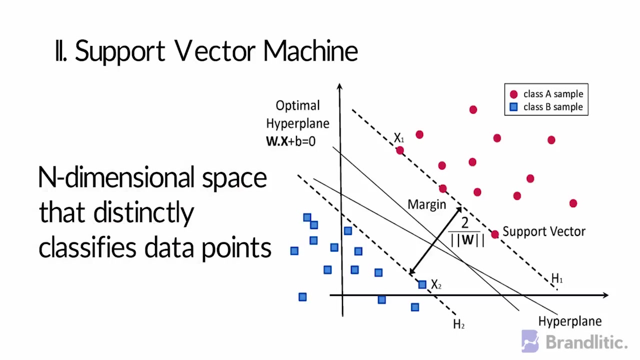 is similar to linear regression but is used to model the probability of a finite number of outcomes, typically two. next support vector machine. it is a supervised classification technique that carries an objective: to find a hyperlain in n-dimensional space that can distinctly classify the data points. next name: base. it's a classifier which acts. 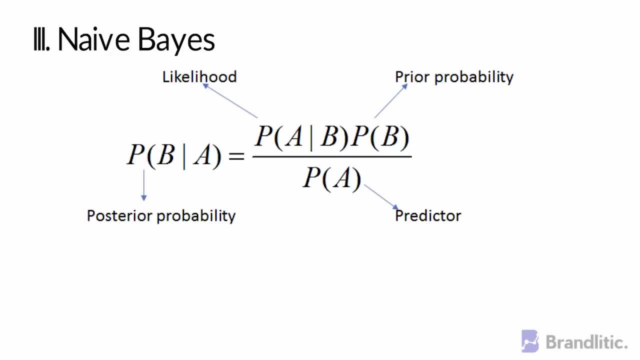 as a probabilistic machine learning model used for classification tasks. the classifier is based on the Bayes theorem. coming up next decision trees, random forests and neural networks. these models follow the same logic as previously explained. the only difference here is that the output is discrete rather than continuous. now, next, let's jump over to unsupervised learning. 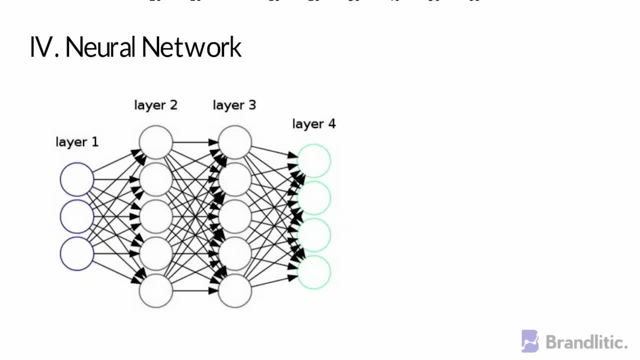 like the neurons in our brain. the circle represents a node, the blue circle represents an input layer, the black circle represents a hidden layer and the green circle represents the output layer. each node in the hidden layer represents a function that input goes through, ultimately leading to the output in the green circles. next classification, so with: 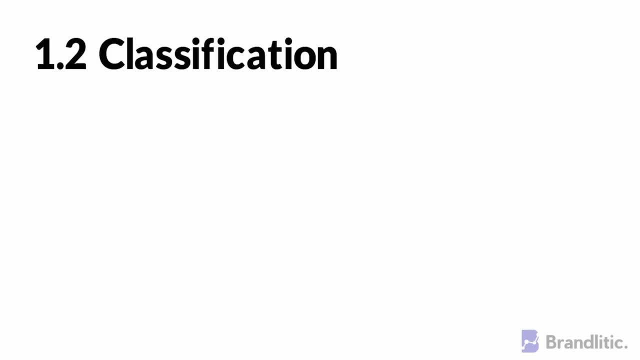 regression types being over, now let's jump to classification. so in classification, the output is discrete. some of the most common types of classification models include: first, logistic regression, which is similar to linear regression but is used to model the probability of a finite number of outcomes, typically two. 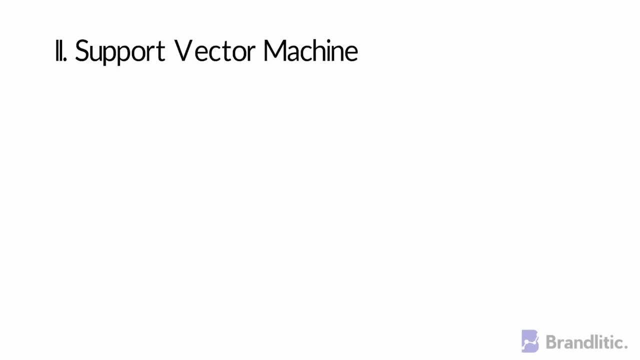 next support vector machine. it is a supervised classification technique that carries an objective: to find a hyperlain in n dimensional space that can distinctly classify the data points. next name: base. it's a classifier which acts as a probabilistic machine learning model used for classifying the data points. the crux of the classifier is based on the bayes theorem coming 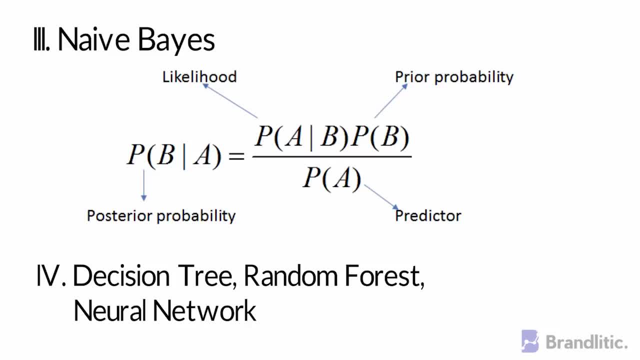 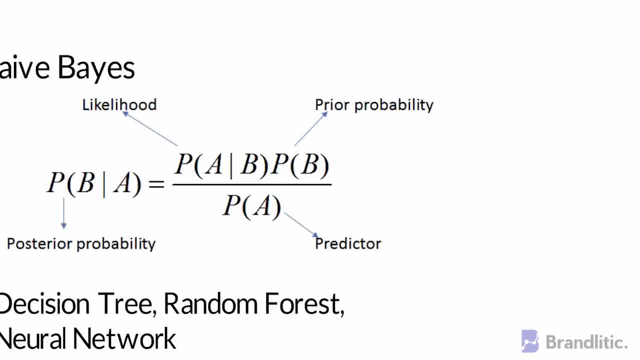 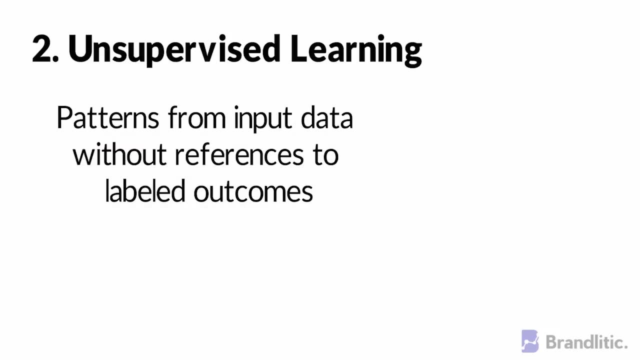 up next decision trees, random forest and neural networks. these models follow the same logic as previously explained. the only difference here is that the output is discrete rather than continuous. now, next, let's jump over to unsupervised learning. unlike supervised learning, unsupervised learning is used to draw inferences and find patterns from input data, without references to the labeled. 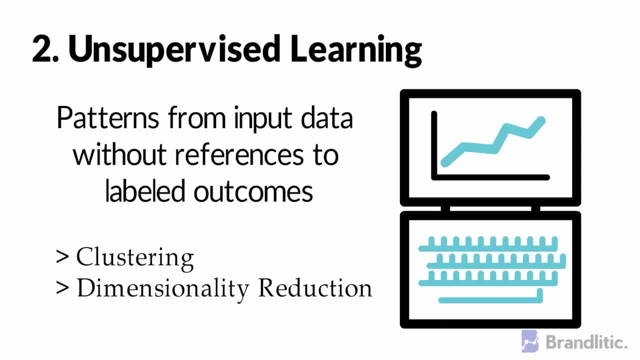 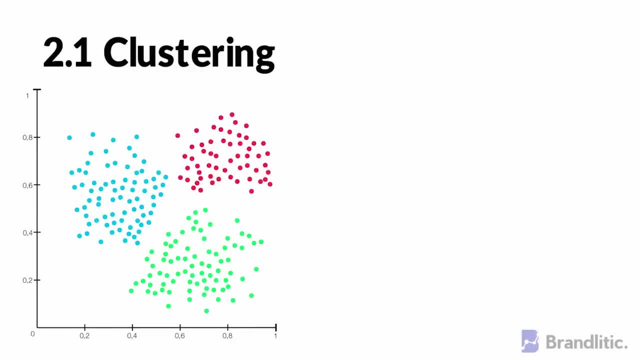 outcome. unsupervised learning includes clustering and dimensionality reduction. clustering involves grouping of data points. it's frequently used for customer segmentation, fraud detection and document classification. common clustering techniques include k-means clustering, hierarchical clustering, mean-shaped clustering and density-based clustering. while each technique has different, 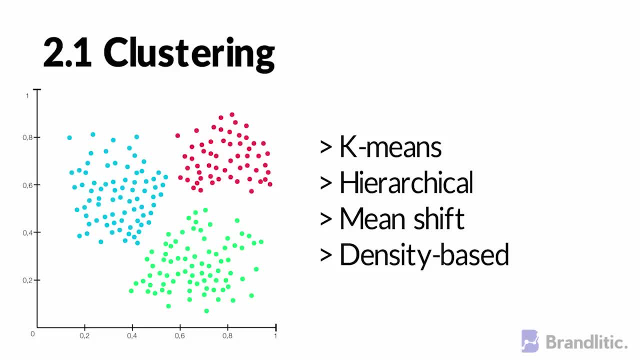 methods in finding clusters. they all aim to achieve the same thing. coming up next: dimensionality reduction. it is a process of reducing. Thank You for watching. Please Subscribe, Like, Share and Comment. Thank you for watching. If you enjoyed this video, please share it with your friends and friends. Thanks for watching, Bye, Bye.